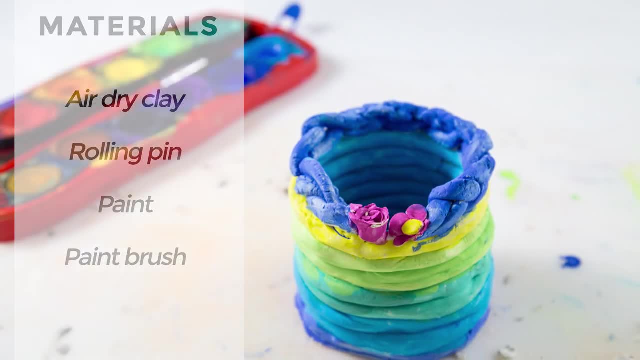 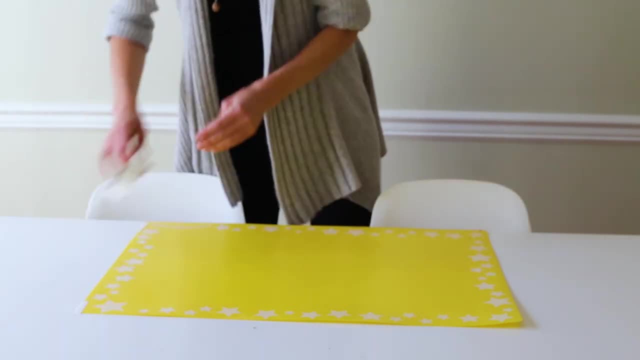 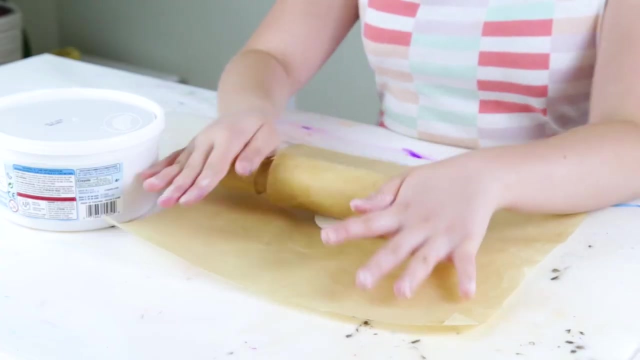 And we will need a paintbrush. A little tip: before creating clay coil pots, Try working on a plastic placemat. This will help protect your work surface. Let's create. We'll start by creating a round cookie out of clay to use as the base of our pot. 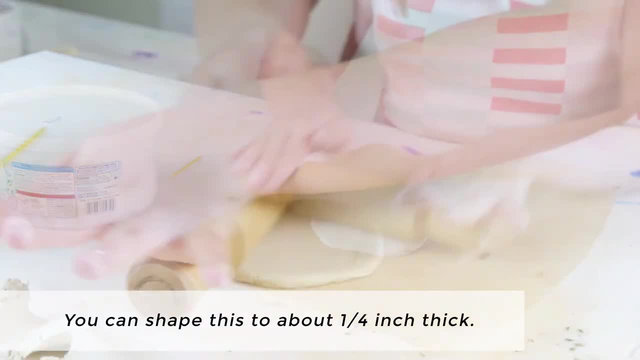 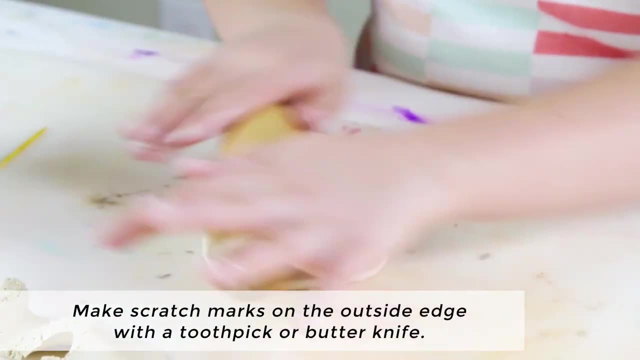 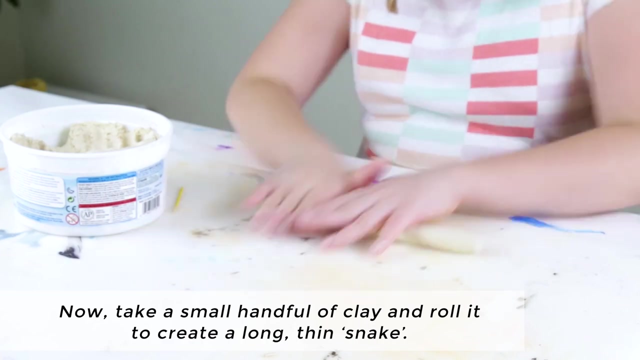 You can shape this by hand or roll it out with a rolling pin to make about a quarter inch thick. Make scratch marks on the outside edge with a toothpick or butter knife. Now we'll take a small handful of clay and roll it between our hands and the table to create a long, thin round cookie. 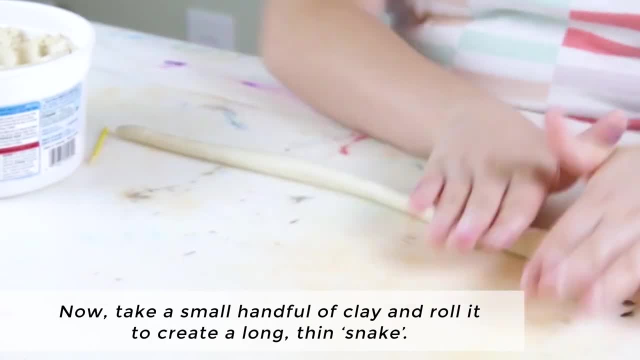 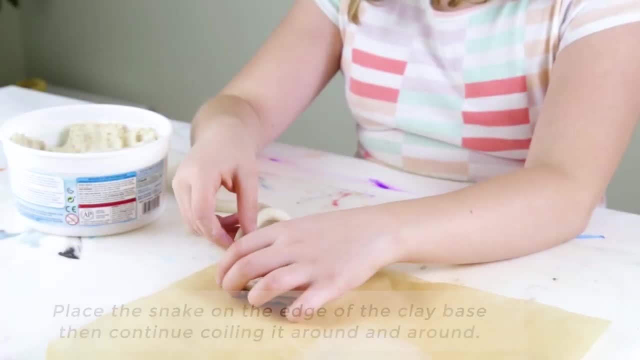 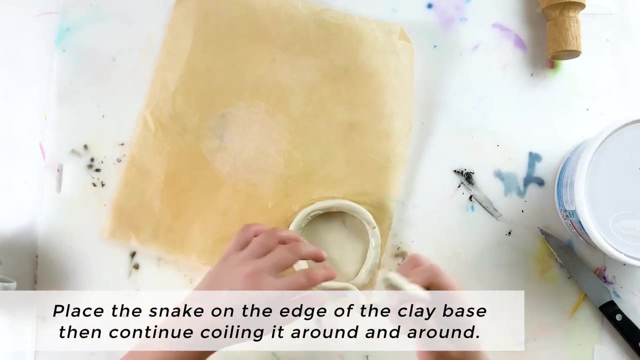 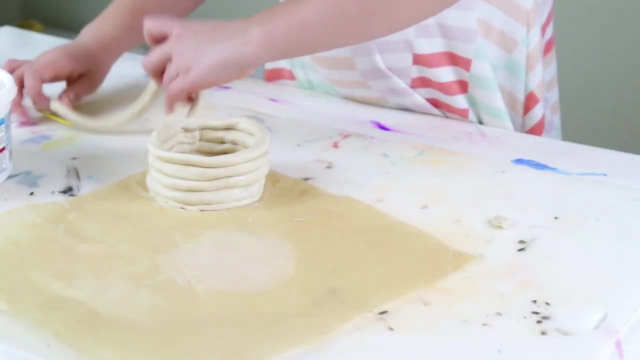 And our guy is ready, We'll crop the edge by rolling the furnaceолог to an extra thiner- Step 10, we'll shape the paint. We'll then attach a stencil to our clay base. You can also use a entersicle to create a long, thin snake. 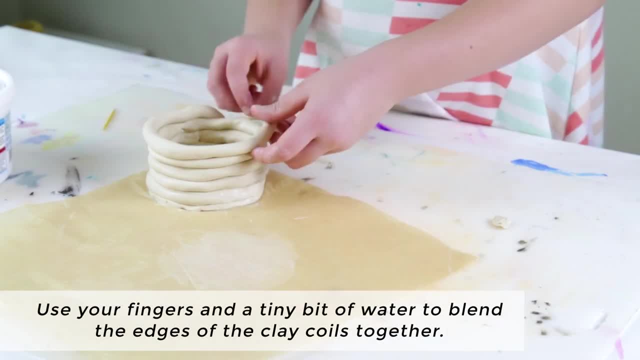 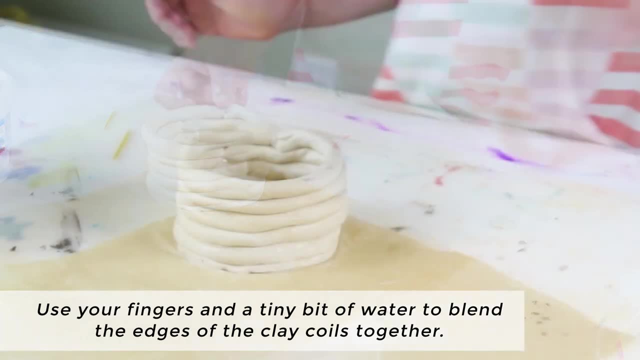 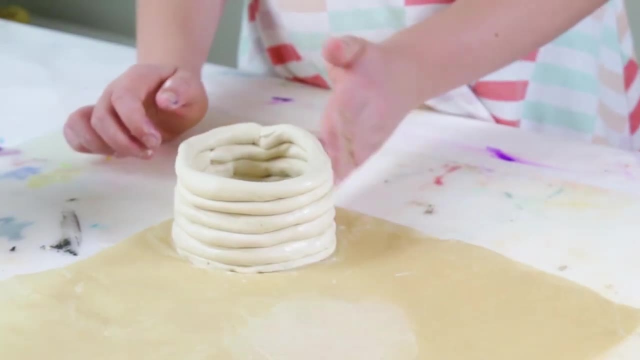 We'll place the snake on the edge of the clay base, over the scratch marks, then continue coiling the snake around and around. Next, we'll use our fingers and a tiny bit of water to blend the edges of the clay coils together a little bit or a lot. 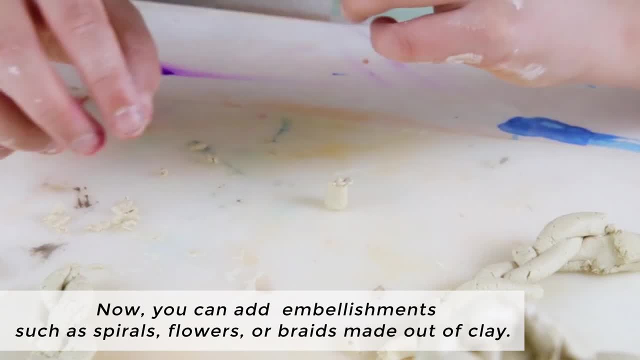 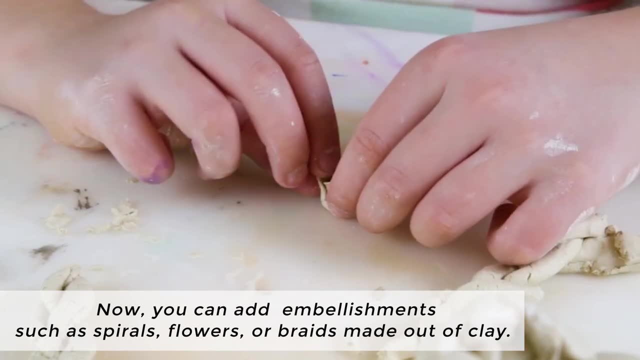 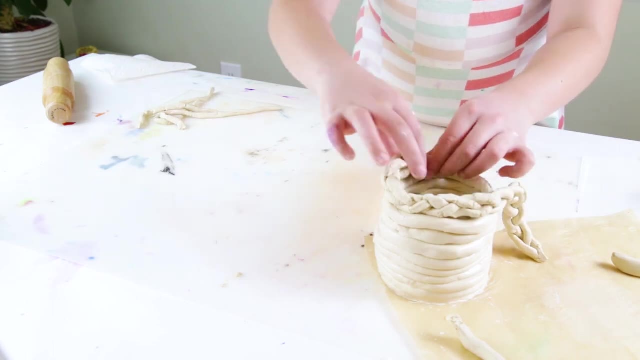 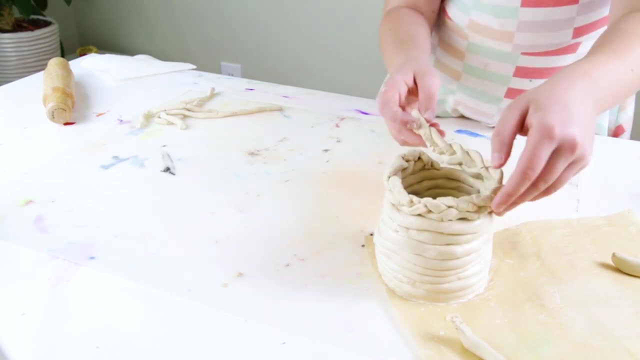 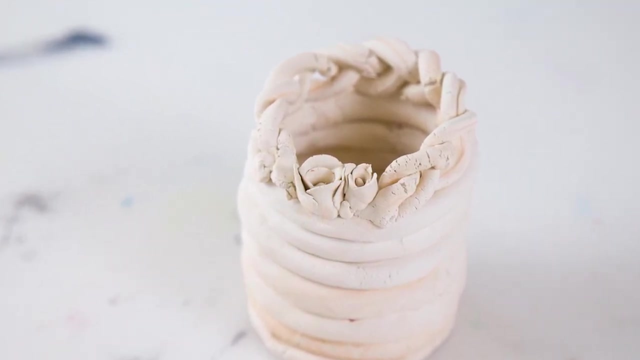 Once you've made your clay coil pot as big as you would like, you can add embellishments such as spirals, flowers or braids made out of clay. Then we'll let our pot dry completely. This can take several days.